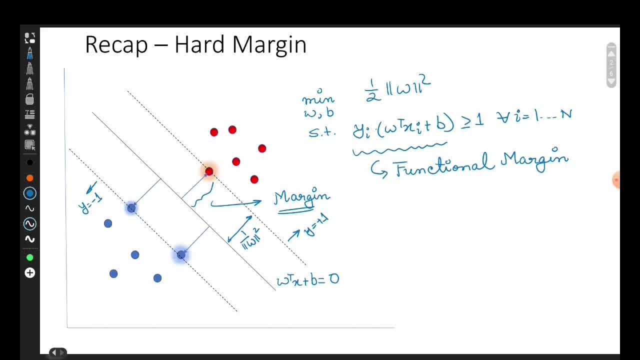 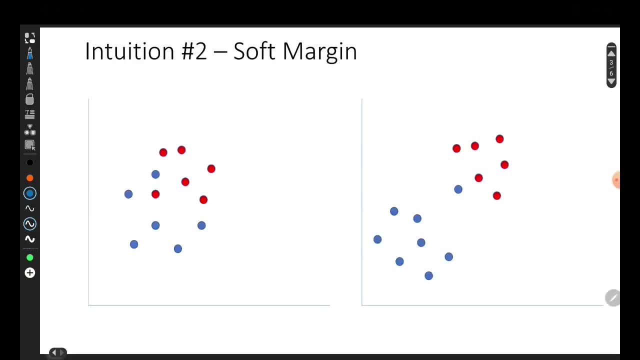 This was a hard constraint that we put on all the points. Now we will see why we might want to relax this constraint. We will look at two cases. The first one is where the data is not linearly separable. So in this case you will not find any hyperplane which can separate all the 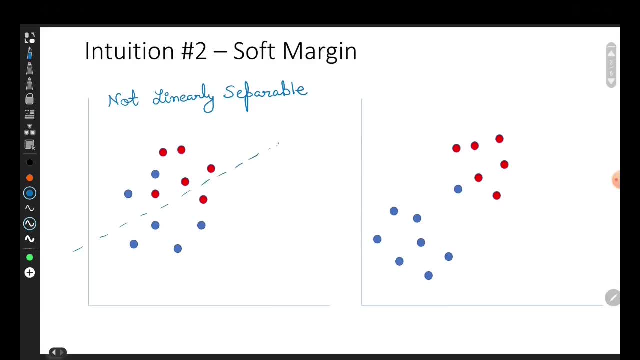 points correctly and therefore will not satisfy the constraint, The functional margin constraint, Hence the hard margin. SVM will not find any hyperplane. Now, if we were to allow some points to be misclassified, then we might find some hyperplane like this, which only does one misclassification, which is of course better than not finding any. 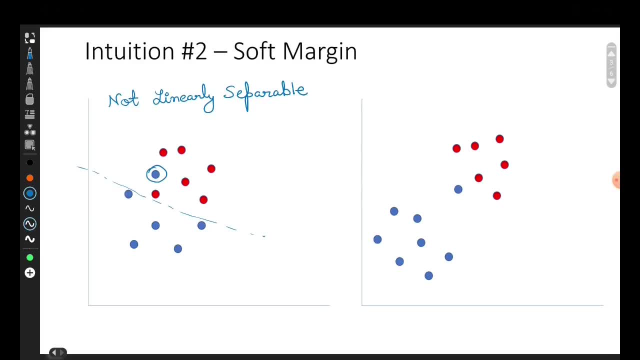 hyperplane at all. In the second case the points are linearly separable, But if you look at this point, this point seems to be an outlier. Now, if all the points must satisfy the functional margin constraint, then the hyperplane that will. 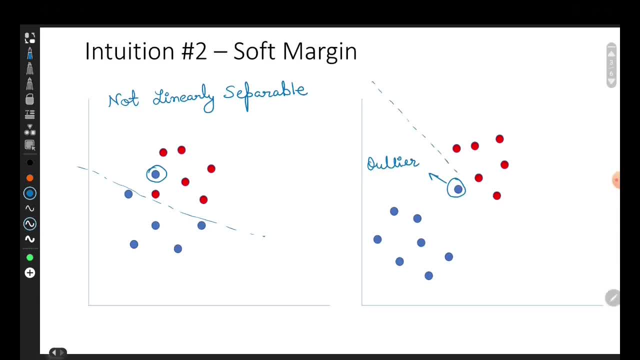 be obtained will be something like this, For which the margin is very small, But hyperplanes such as this, where there are some misclassifications, might generalize better to an unseen example because of the bigger margin. So in this case you might not want, or, kindlyoshima, increase out of the fraction. In this case, the margin of the hyperplane is less than four constant. We might want to stop. you might not need to adjust rescale In the next interventions. we might want to go ahead in flat rather than flat. I am guessing this guy may be right. If you want better than less than one, This point will always be smaller in run to be an outlier. Now, if you would do something like this, it would only win n the 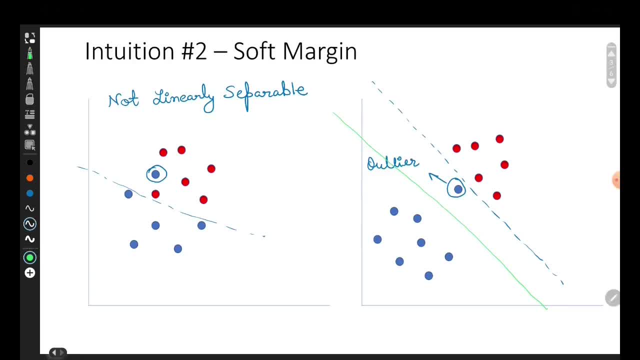 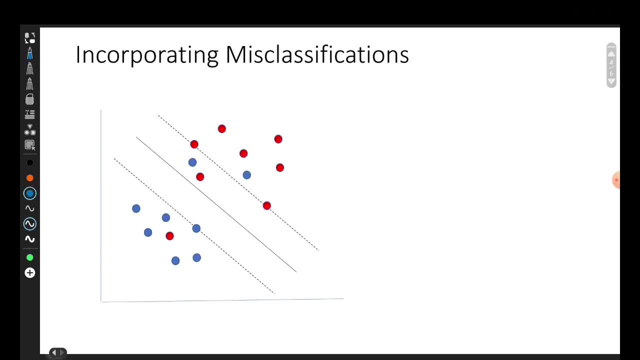 not want to over-fit the data and allow for misclassifications. So now, how can we incorporate misclassifications in our formulation? We can do so by relaxing the functional margin constraint a bit. So let us look at this point which is misclassified. let this point be xi. 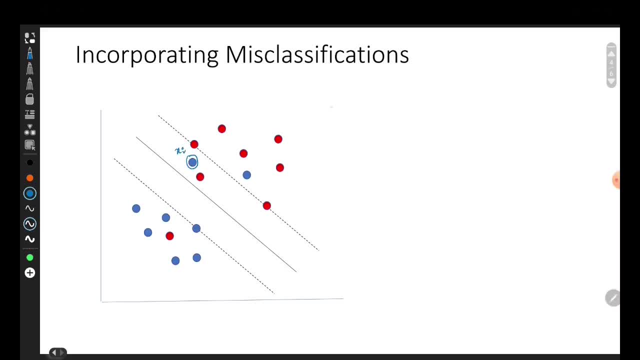 For this point. the functional margin constraint says that yi into w, transpose xi plus b, should be greater than or equal to 1.. But in this case this is not greater than or equal to 1, this is in fact less than 1. 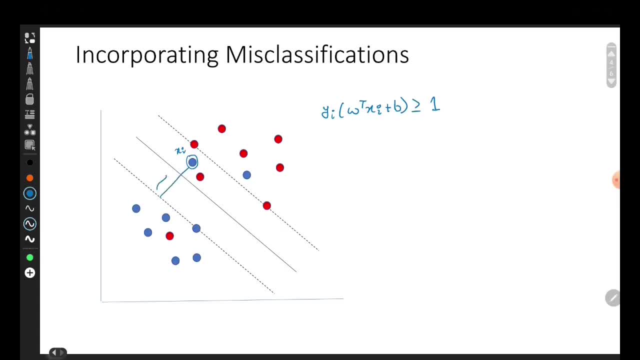 by, let's say, some amount xi i- This should have been 1 and it is less than that- by this amount xi i. so this is 1 minus xi i. The functional margin is 1 minus xi i for this point xi. This xi i gives some slack. 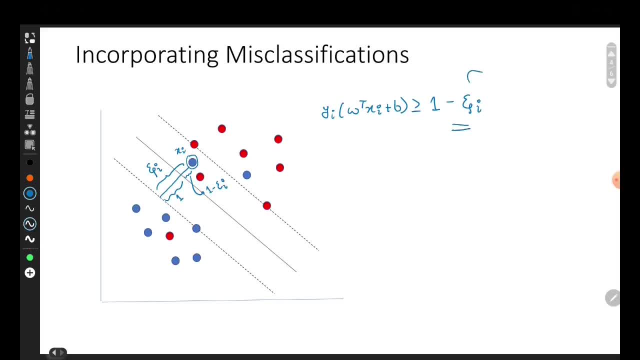 So the functional margin constraint and else is called a slack variable. Xi. i tells us how much error there is for this point. We would have ideally liked this yi into w, transpose xi plus b to be greater than 1, but it is less than 1 by this amount. xi i. 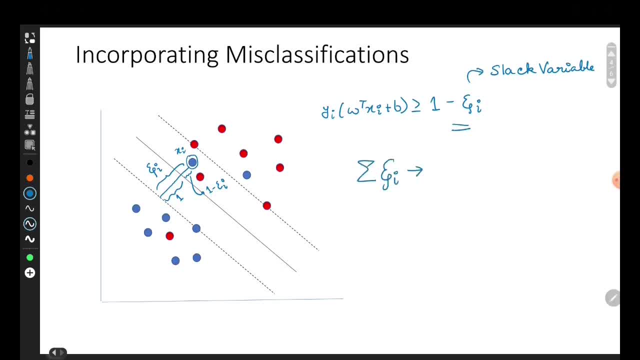 The sum of all xi i's gives us a measure of the amount of error For this hyperplane and for the points which are correctly classified. let's say, for this point xi i, xi j will be equal to 0. This is because we do not want to have any error when the points are correctly classified. 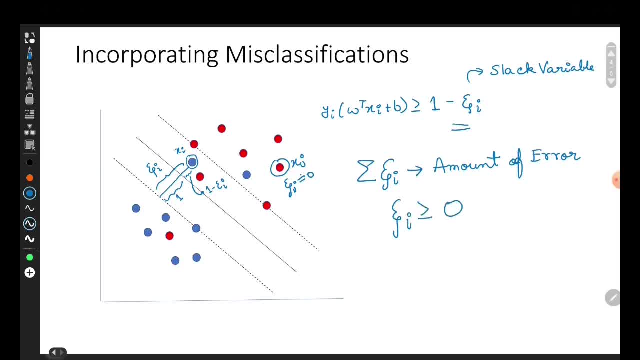 So xi i's should always be greater than or equal to 0.. It will be equal to 0 for points which will have functional margin greater than or equal to 1, and it will be greater than 0 for points with functional margin less than 1.. 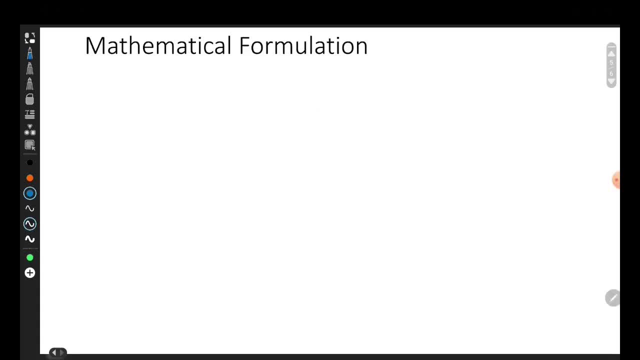 We can now formulate our optimization problem as follows: For the objective we will have minimize half norm w square, and the constraint will now be relaxed using slack variables. So we will have yi into w, transpose xi plus b. We will also have xi i greater than or equal to 1 minus xi i. for all i equal to 1 to n. 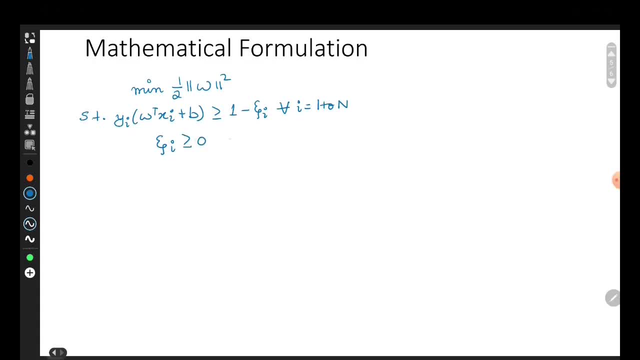 And we will also have xi i greater than or equal to 0 for all i equal to 1 to n. Now, in this optimization formulation we have not penalized the error. So what the optimization algorithm will do is it will set xi i to be greater than or. 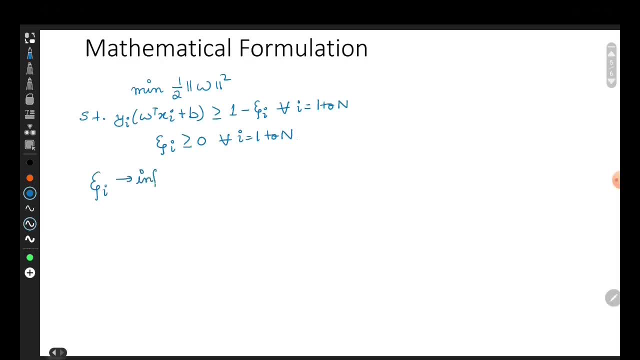 equal to 1 minus xi, i to be infinity, Which will make the constraint yi into w, transpose xi plus b greater than or equal to minus infinity, which is trivially satisfied, which basically means that it will now be just minimizing half norm w square. 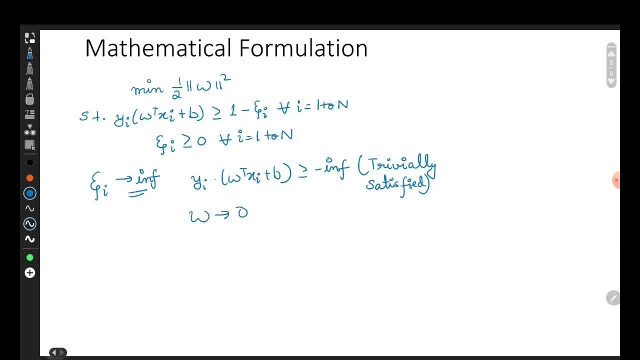 Which will result in w being 0. This basically means that the optimization would ignore the data completely and will focus on making this w 0, which we don't want to happen. So what we are going to do is we are going to add some penalty for these errors by minimizing. 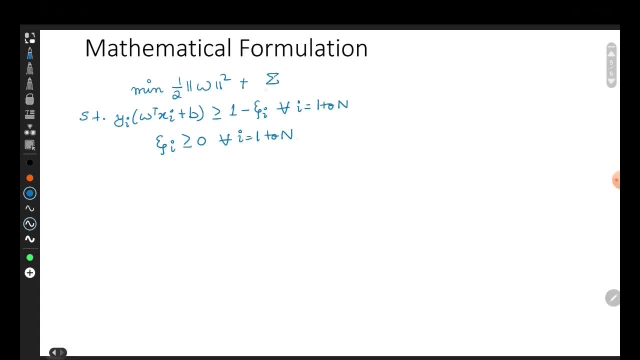 along with half norm w square sum over i equal to 1 to n, xi, i, And we will also have hyperparameter term here, c, whose job is to basically control the trade-off between maximizing the margin, which is this term, and maximizing the margin, which 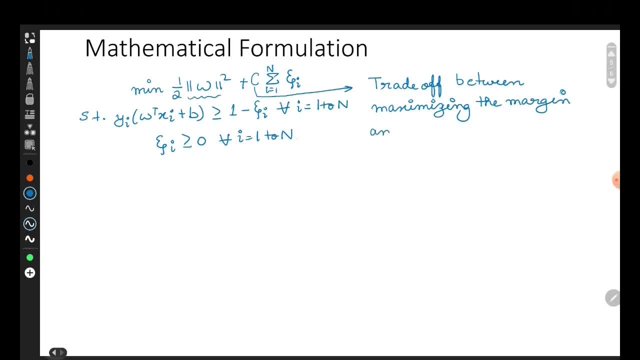 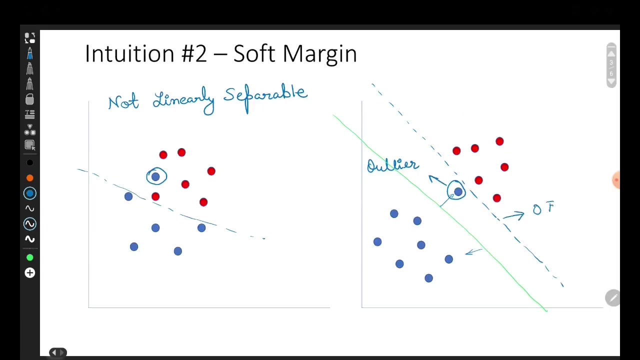 is this term, And minimizing errors, which is this term. Now we have already seen before the trade-off between maximizing the margin and minimizing errors. So this hyperplane had zero errors but smaller margin. Now this hyperplane had one error with bigger margin. 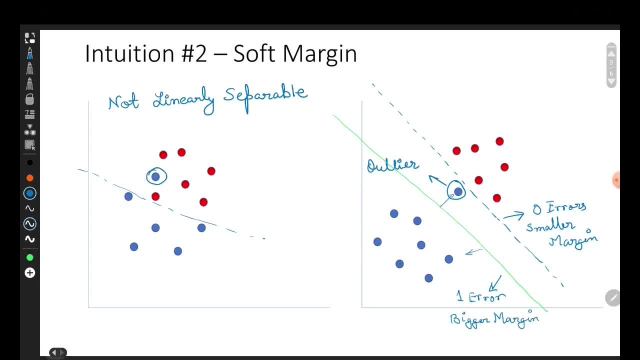 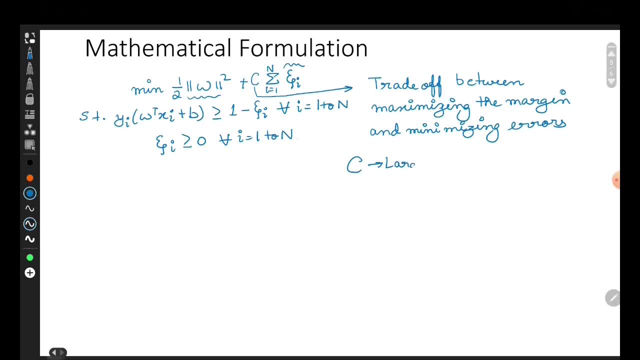 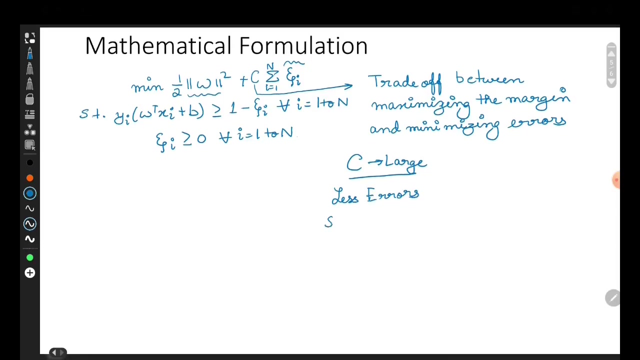 So let's understand this role of c. So if c is large then it is going to give more weight on the errors, So you will have less errors but your margin will be small, so you have smaller margin. If c is small, that means it will give weightage to the half norm w square more, which basically 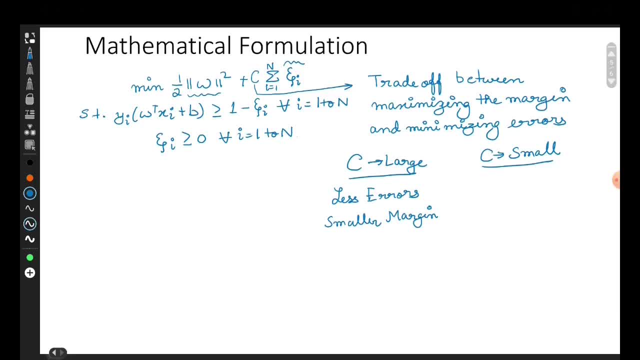 means it will focus more on maximizing the margin and less on number of errors. So you will have more errors but bigger margin as well. Now, if we look at the two extreme cases, the first one will be c equal to zero. So we have already looked at this case. 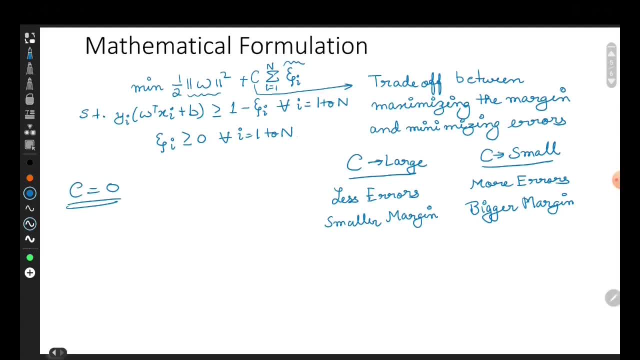 This basically means there is no penalty for errors, And what is going to happen is xi i's will be very large. So we have already looked at this case. This basically means there is no penalty for errors, And what is going to happen is xi i's will be very large. 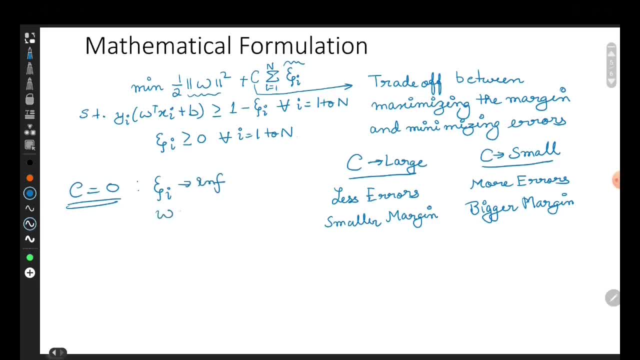 So we have already looked at this case. This basically means there is no penalty for errors, And what is going to happen is xi i's will be very large, So we have already looked at this case. This basically means there is no penalty for errors. 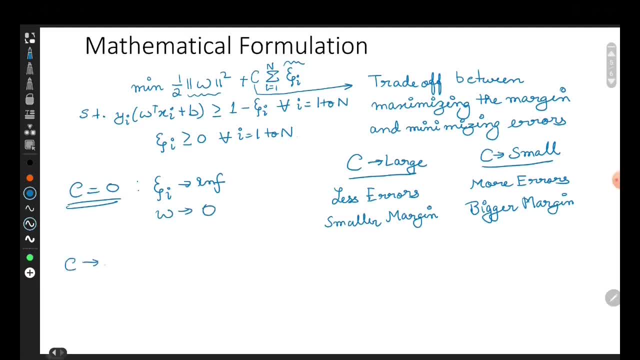 And what is going to happen is xi i's will be very large. So we have already looked at this case. This basically means there is no penalty for errors, And what is going to happen is xi i's will be very large. So we have already looked at this case. 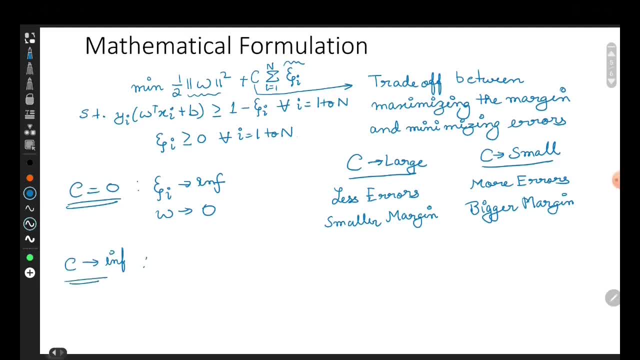 This basically means there is no penalty for errors, And what is going to happen is xi i's will be very large. So we have already looked at this case. This basically means there is no penalty for errors, And what is going to happen is xi i's will be very large. 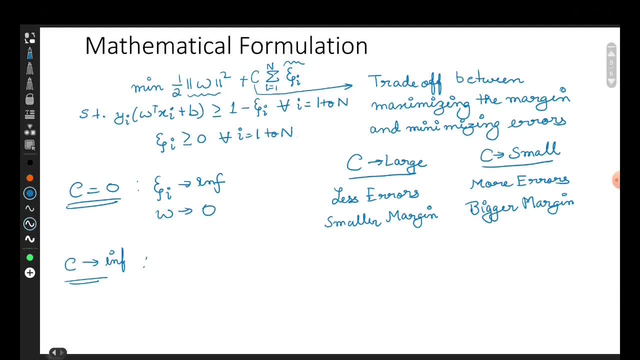 So we have already looked at this case. Then, to reduce your objective function, it basically needs xi i's to be 0, otherwise the objective will be infinite. So xi i is 0 means there will be no errors, which would imply that the functional margin 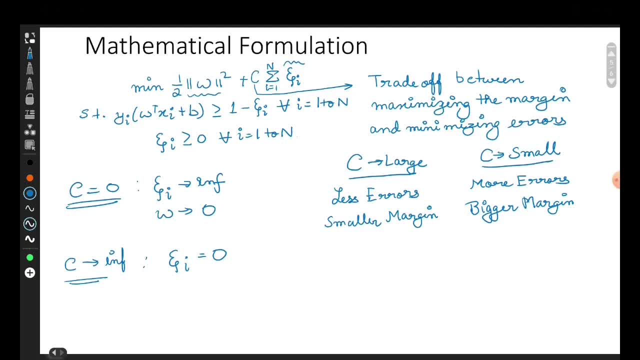 constraint yi into w. transpose xi plus b greater than or equal to 1. holds true for all the points, basically implying that w will converge to a w. hard margin SVM. So this is basically equivalent to the hard margin formulation of SVMs. Now let us look at these constraints. 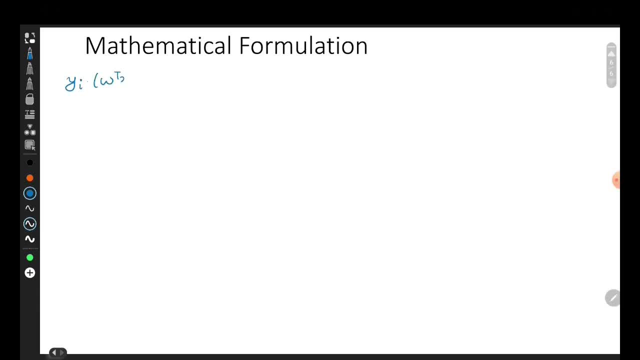 The first constraint was: yi into w. transpose xi plus b is greater than or equal to 1.. Now we can rewrite this constraint as: xi i is greater than or equal to 1 minus yi into w. transpose xi plus b. The second constraint was xi i is greater than or equal to 0.. 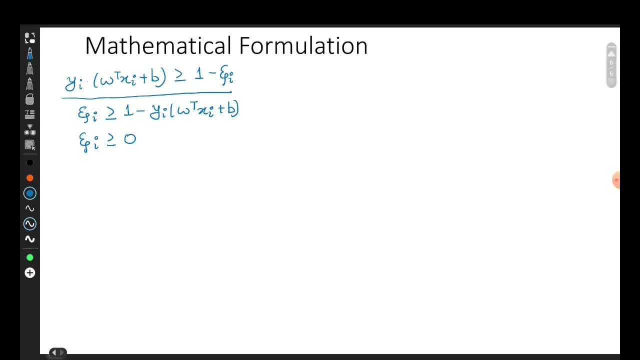 Since we are trying to minimize xi i. therefore for the optimal value of xi i we have to have xi i star. One of these inequalities needs to be tied. Why is that? Because if the optimal value xi i star is greater than both these terms, then we could. 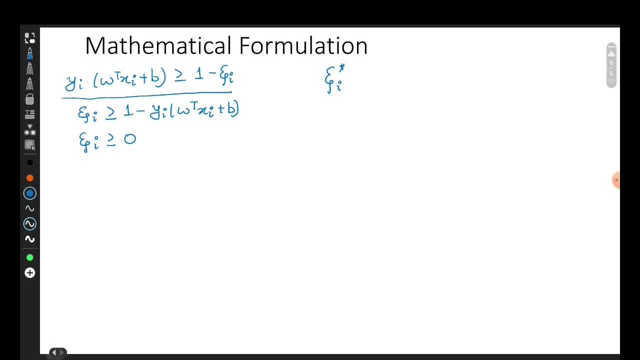 reduce xi i star by some amount delta, which will decrease your optimization objective without violating the constraints, which cannot happen. So one of these inequalities must hold. Which one will it be? It will be the one with the larger quantity, Because it needs to satisfy both the constraints. 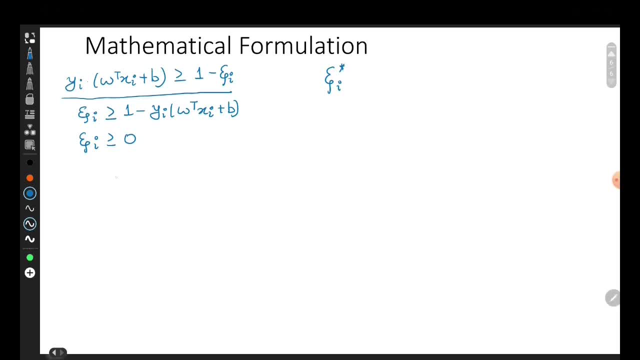 Why is that Say? for example, if you have to enumerate x, x greater than or equal to 2 and x greater than or equal to 3,, then the smallest value of x which will satisfy both the constraints will be x equal to 3, which is the larger of the two values, right? 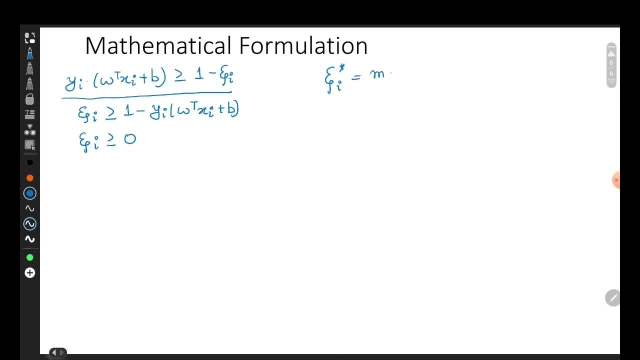 So we are going to have xi i star equal to max of 0 comma 1 minus yi into w. transpose xi i plus w star. transpose xi i plus b star. Now, knowing this, we can rewrite our objective function and we will move the xi i as follows: 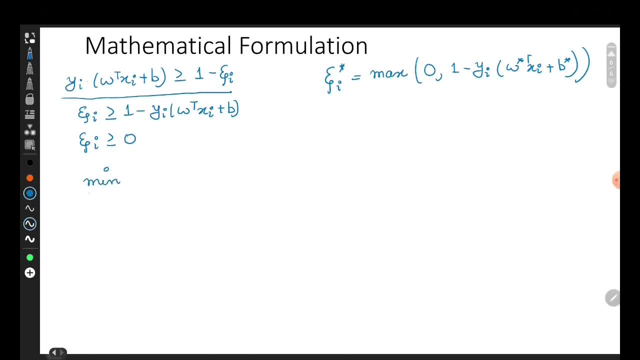 that we will have. minimise what W and B is: 1 x 1 x, 1 x 2 x. prime of W: the half norm w square plus c x. sum over i equal to 1 to n of xi i. we will write max of 0 comma, 1 minus y i into w. transpose xi plus b. 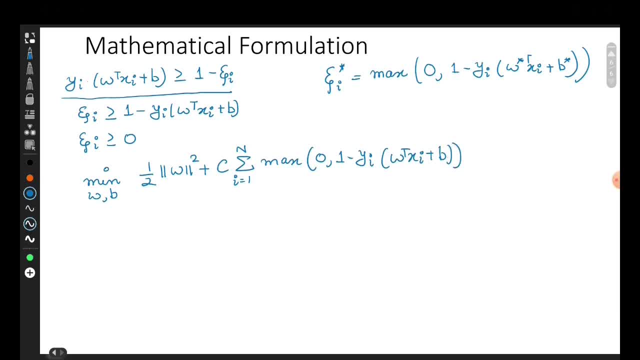 Now this is the final form for the optimization problem of soft margin SVMs. This term here max over 0 comma. 1 minus y i into w, transpose xi plus b: this is called hinge loss. Let us try to understand what this loss is exactly doing. 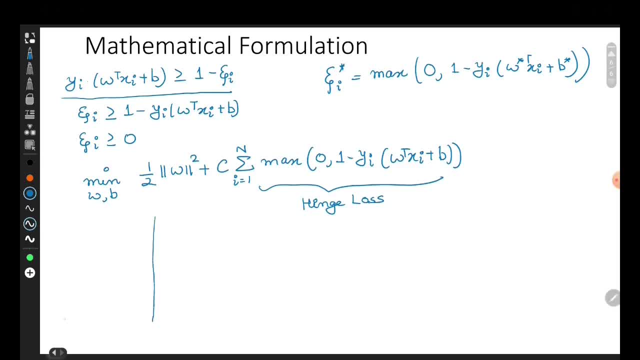 So we can plot a graph here where the x axis will be y i into w, transpose xi plus b, and the y axis will be the hinge loss. So when this y i into w transpose xi plus b is 1 or greater, Then the value of the loss will be 0.. 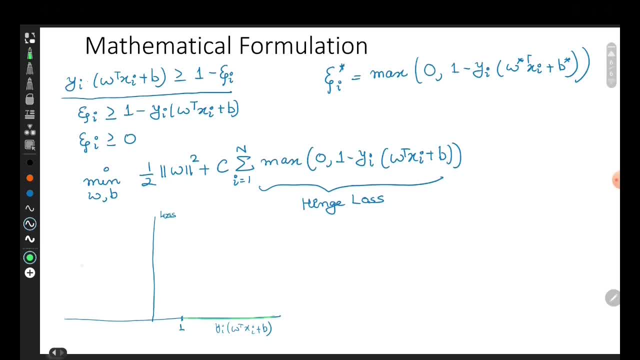 And when the value is less than 1, then it is going to be 1 minus y i into w, transpose xi plus b, which will look something like this: This is 1 minus y i into w, transpose xi plus b. So this loss penalizes whenever the functional margin is less than 1.. 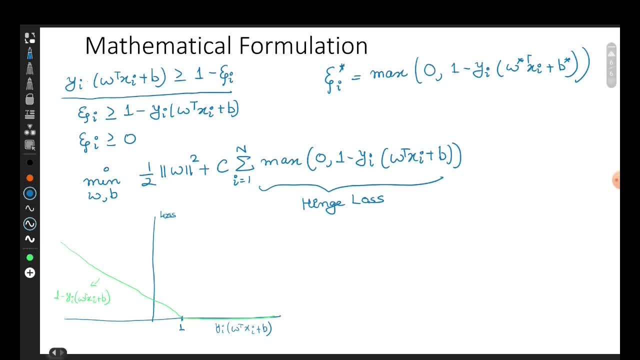 So this loss penalizes whenever the functional margin is less than 1.. And the amount by which it penalizes is equal to its difference from 1.. Now, another way to look at this objective function is to think of it as minimizing the hinge loss plus, some lambda times, the regularizer over w, where the regularization is l to 0.. Now, another way to look at this objective function is to think of it as minimizing the hinge loss plus some lambda times the regularizer over w, where the regularization is l to 0. And this lambda plays the role of 1 by c. And this lambda plays the role of 1 by c. 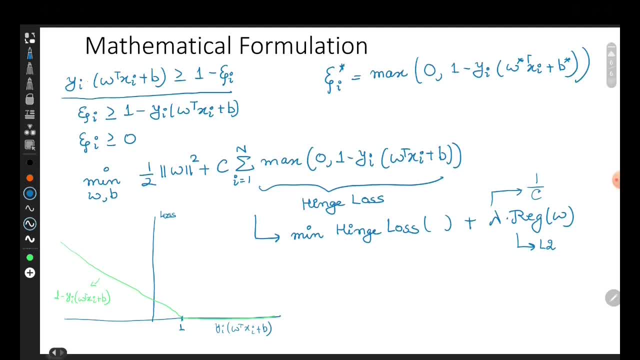 So this is all about soft margin SVMs. So this is all about soft margin SVMs. There is another concept about SVMs, which is kernels, which we will discuss in another video. In the next video we will look at how we can use scikit-learn for doing classification. 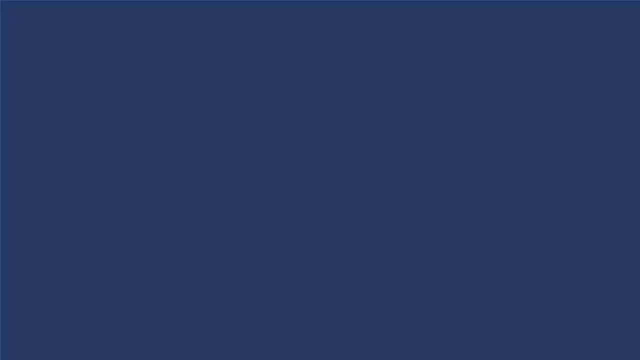 using SVMs. So see you in the next video. Bye-bye.